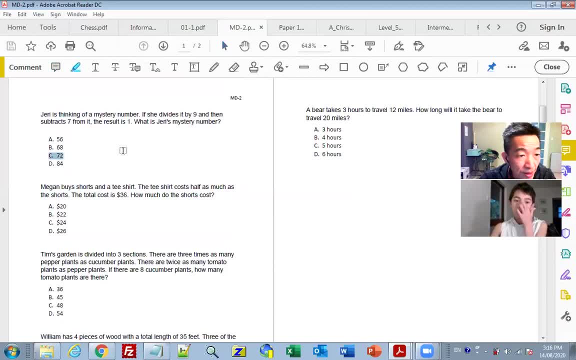 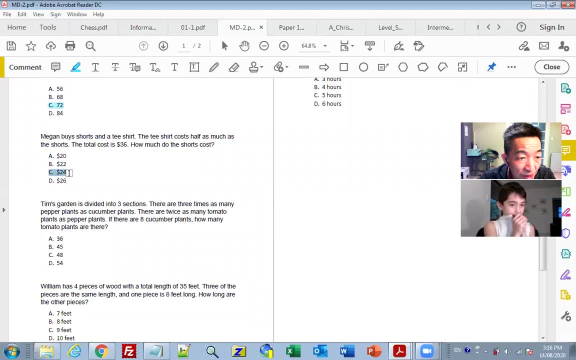 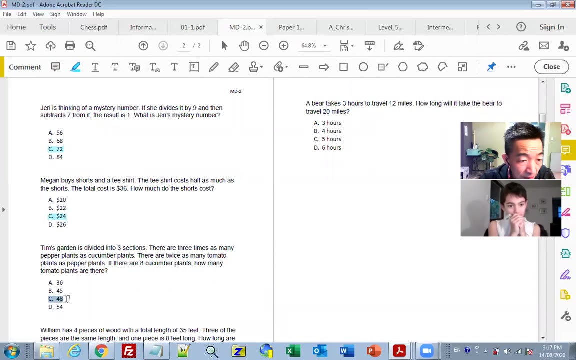 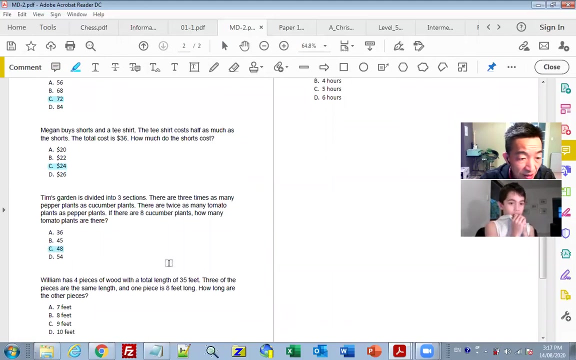 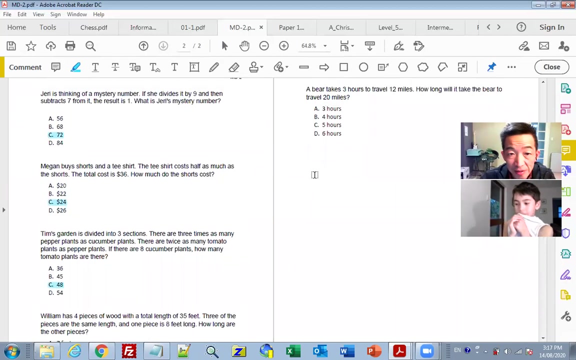 72C, Question number two: 24.. Good, Question number three: 48.. 48.. Okay, Question number four: Nine foot. Okay, Yeah, Last question. Yeah, Number five, Five hours. All good, Okay. 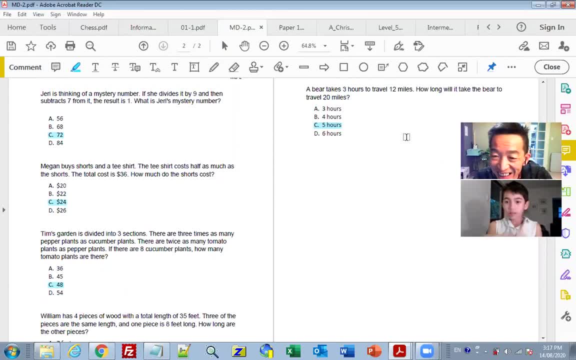 100% correct. All right, Okay, Can you just- let's go back to from the first question- just briefly explain to you what do you do? Yeah, Yeah, Okay, Okay, How did you find 72?? Well, so I gave mystery number X, So it was X divided by nine. 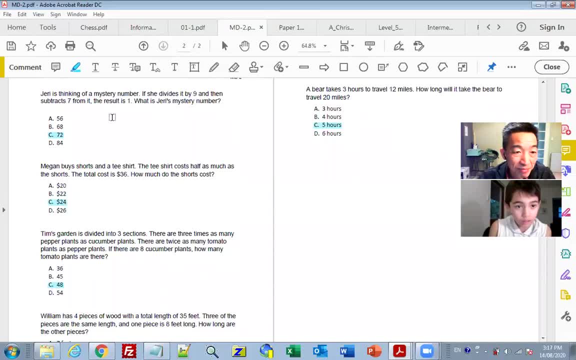 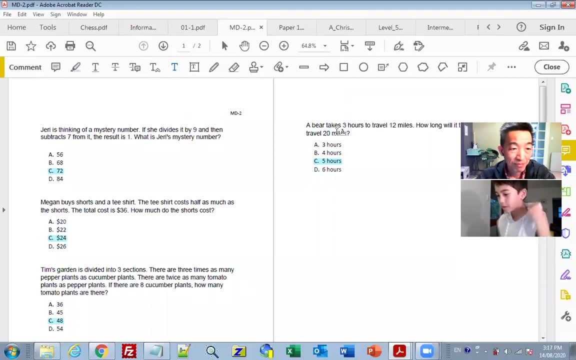 minus seven equals one. So I use 72 divided by nine, which equals eight. Eight minus seven equals one. Yeah, Divided by nine, and then up to seven from it: Yeah. So we work backwards right, Starting from the result One, and we're invert the operations: Yeah, And the one by one. 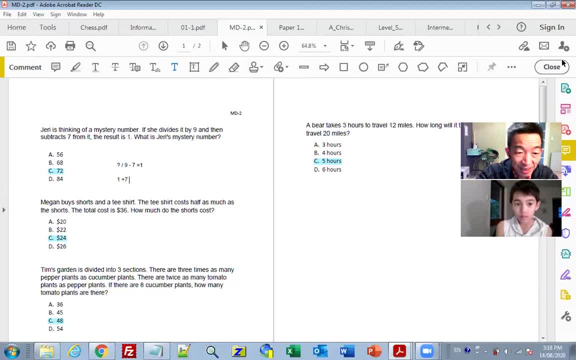 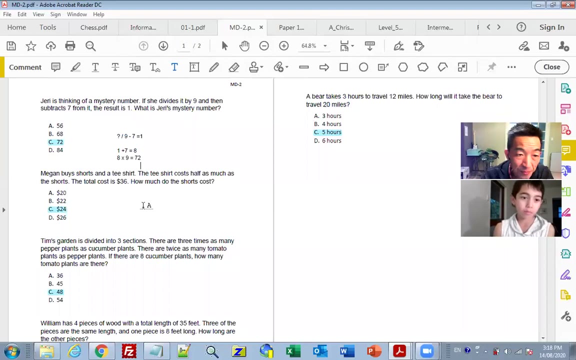 Yeah, So we plus seven. first, Let's look at it, Yeah, And then eight times nine, Yeah, yeah, yeah, get a 72. good job, okay, uh. second question: yep, uh, we can buy shorts in the tea. the tea costs half as much as the. 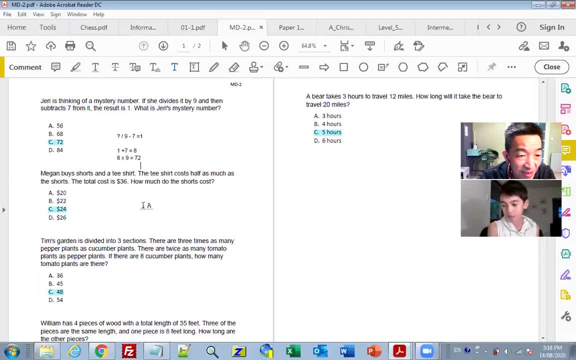 shorts, the total cost is 36. how much do they cost so? so shirt equals half times y, so half of the, so they spend 36. so you got to figure out how much the half of them would half would cost, so that so you would have to do 27 divided up. 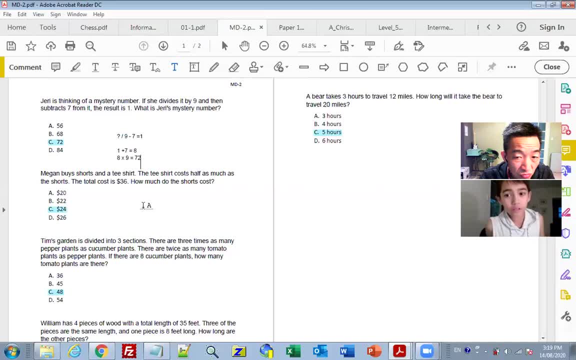 you would have to do 36 divided by 3, which is 12.. very good, the t cost 12, so that's 12 times yeah, so it costs 24.. yeah, yeah, okay. so if we just uh, yeah, okay, and that the if we say t-shirt is the one part, i think 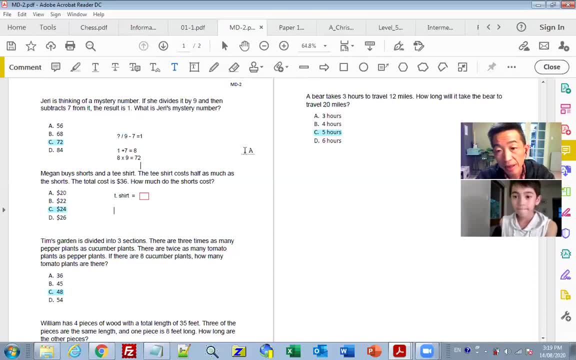 that we we're going to use uh a part. yeah, okay, it's not a real unit of measurement, but it is very uh pro have to prove it to be very efficient, useful, uh, when you think that's how you buy a shirt you sit for those selective exams. All right, It's the. we just say what t-shirt is one. 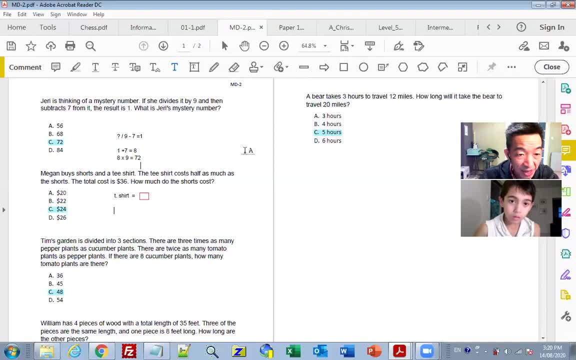 part the price, So the shorts, since it has the double of the price of the t-shirt. Yeah, So we can say the price of a short is two parts. Okay, We'll just say this: one Yeah Plus Yeah To pass. Yeah, Okay, Yeah, Okay. So all together is that the we have a $36.. 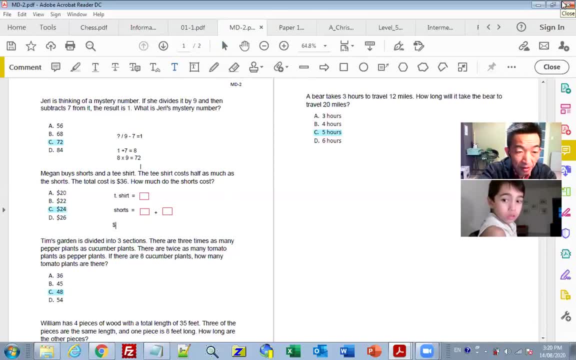 So it's the yeah. It's consist of how many? Three times This is the three times this, three times to pass: Yeah, Three parts all together. Okay, So there are four. we just say Yeah, So we can get the the size of the part. Yeah, Yeah. 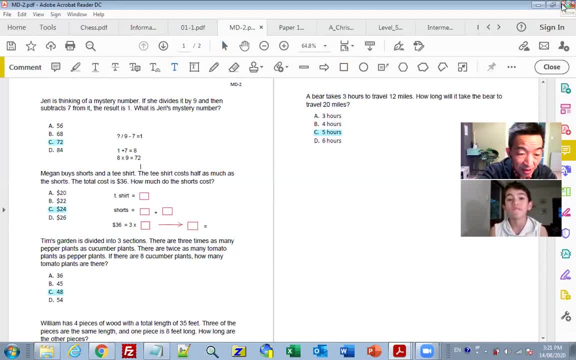 Yeah, Okay, We have the $12.. Correct: Yeah, Yeah, Of course Yeah, Then we go back to shorts. That is the will give us Yeah, So is the answer is Yeah. 12 times two Get us $24.. 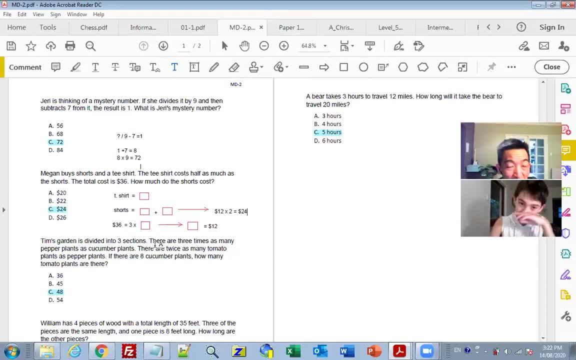 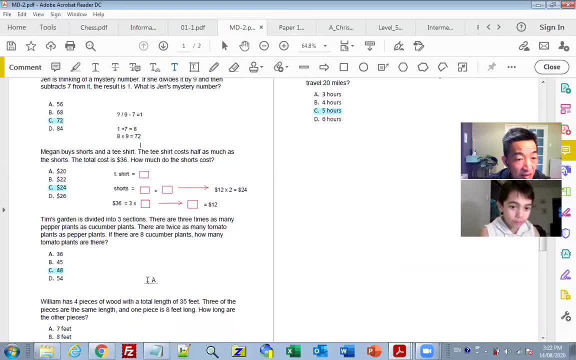 Tim's garden is divided into three sections. There are three times as many pepper plants as cucumber plants. There are twice as many tomato plants as pepper plants. If there are eight cucumber plants, how many tomato plants are there? So it tells you that there's eight cucumber plants. Okay. 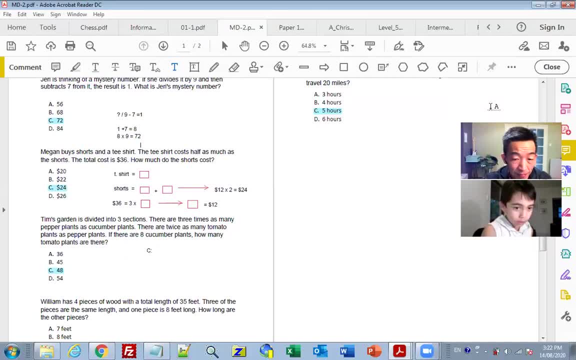 There's three, there's three times as many pepper plants, So that's eight times three, Eight times three, which is 24, and 24 times two is 48.. Yeah, Okay, So it's cucumber plants that we have eight. Yeah, Yeah. 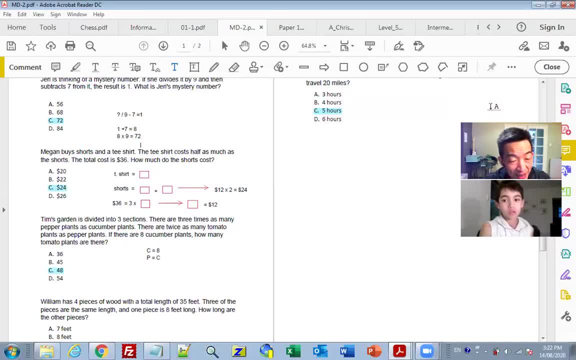 So the pepper plants is the cucumber plants times three. Yeah, Times three, get us 24.. And tomato plants is the pepper plants times three. And tomato plants is the pepper plants times two, 48.. 48.. Very good, Okay. Next. 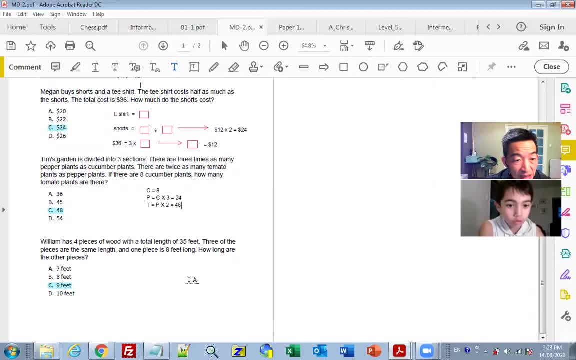 William has four pieces of wood with a total length of 35 feet. Three of the pieces are the same length and one piece is eight foot long. How long are the other pieces? So you take away eight from 35.. Mm-hmm. 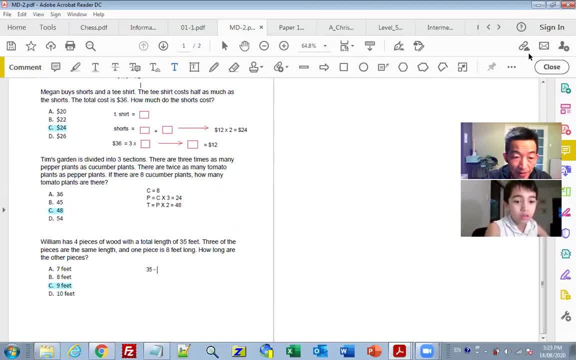 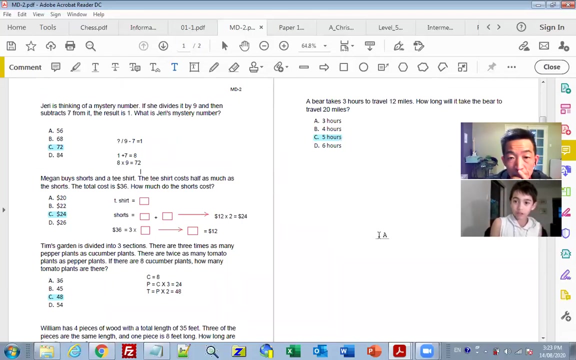 With 27.. Yeah, And then 27 divided by the next three parts is nine, So the three of the parts are nine feet long. Yeah, Okay, Good, Good. Last question: Yeah, A bear takes three hours to travel 12 miles. How long will it take the bear to travel 20 miles?